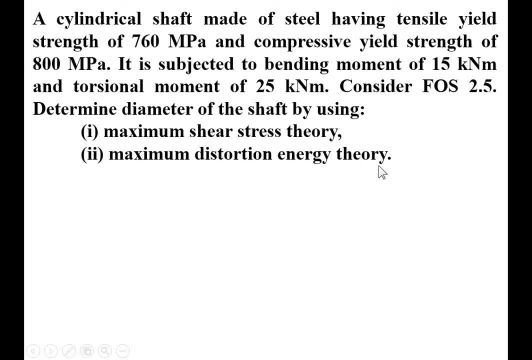 shear stress theory and maximum distortion energy theory. So first of all try to understand the given description with the help of figure. So let's take the cylindrical shaft and that is subjected to torsional moment of 25 kilonewton into meter. So this is the neutral. 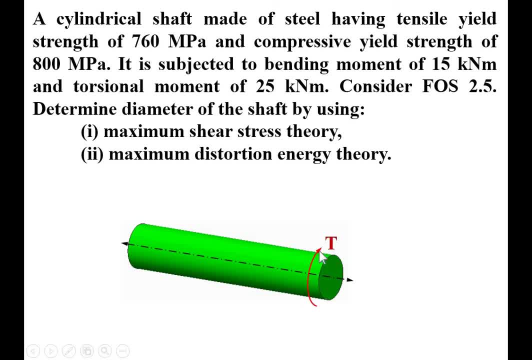 axis and that is subjected to the torsional moment T at the two ends in opposite direction. So this is T in the opposite direction, So that is subjected to torsional moment. It is also subjected to bending moment, So you can say: this is the bending moment M. 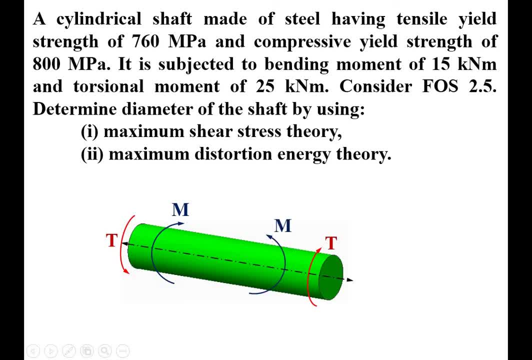 in opposite direction. So the cylindrical shaft is subjected to both twisting moment as well as bending moment, and so that you have to apply different theories of failures. So now we have to find the diameter of this shaft that is subjected to the twisting moment as well as. 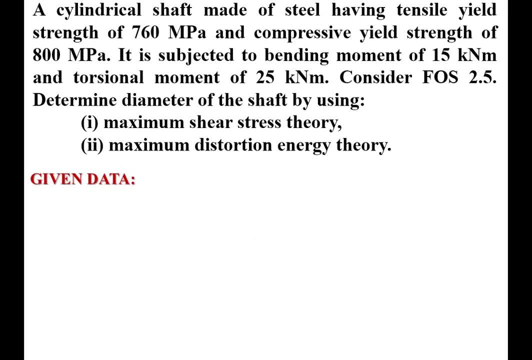 bending moment. First of all, write down the given data So that is given to you. So the principal portion of the torsional moment is 15 kilonewton into meter. torsional moment that is T, 25 kilonewton into meter, and we want to find the shaft diameter. 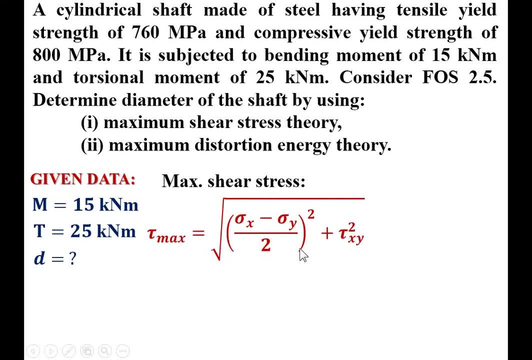 So D is equal to question mark. You know that maximum shear stress, tau max, is equal to this. Here the shaft is subjected to bending, so that you will get sigma x, we will get shear stress, stress in y direction is not developed, and so that you can say sigma y is. 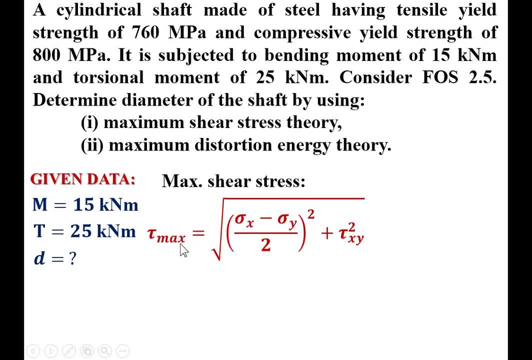 equal to zero. so if you want to find the maximum shear stress, then you have to find the sigma x. we have to find the sigma y, but that you know that is equal to zero, and you have to find the tau. so if you put it over here, sigma y is equal to zero, then your tau max is this one. 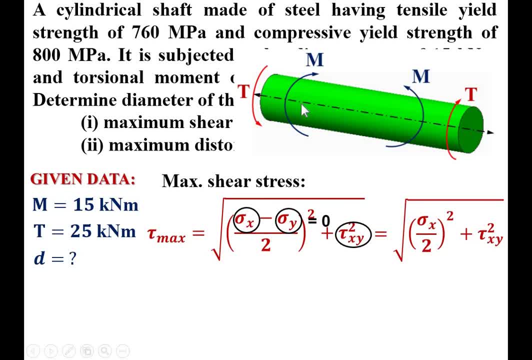 so due to the bending moment, the stress produce is perpendicular to this cross section and so that you can say it is x direction. so the stress produced due to the bending moment is called as sigma x and due to the twisting moment that means torque the stress, Charlotte. 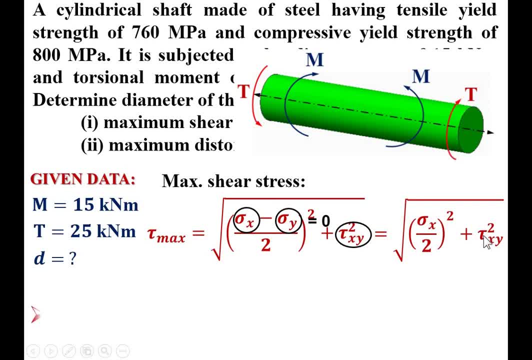 the bending fraction variably is called a Radian feed and so that it is bind to the buchrach speed, shear stress is produced and that you can say tau. so i can use the fundamental equation of bending moment: m by i is equal to sigma by y, where sigma is the bending stress. so i can say bending moment. 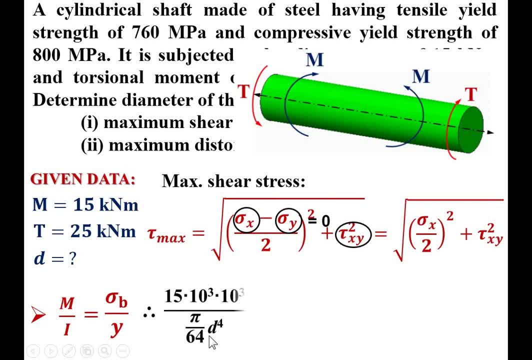 is given to you 15 kilo newton into meter, so i can say: 15 kilo newton that means 10 raised to 3 meter. that means 10 raise to 3 mm divided by i, that means moment of inertia of the circular cross section and as you know that it is pi by 64, d raise to 4. 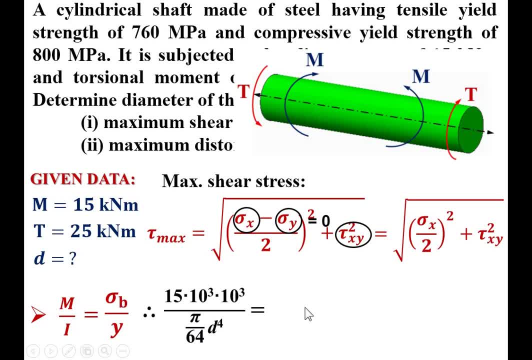 is equal to sigma b. that is the bending stress that i want to find upon y. that is the distance from the neutral axis to extreme fiber, and that is what d by 2. so if you simplify this equation then you will get sigma b in terms of diameter. so sigma b is equal. 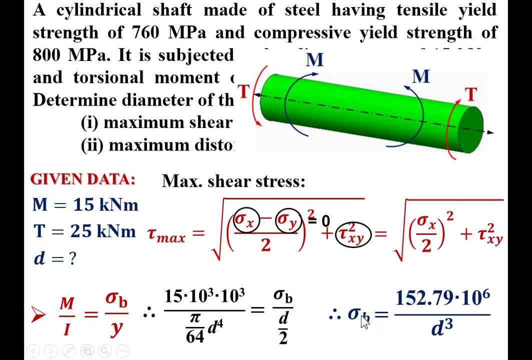 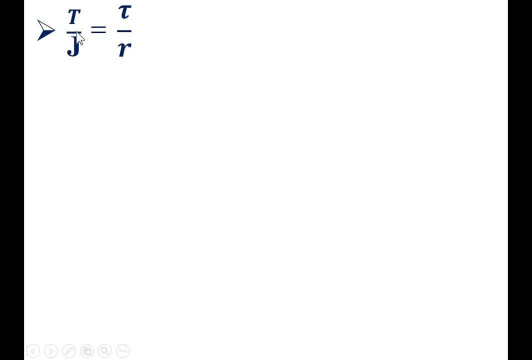 to this one and that sigma b is nothing, but it is what your sigma x, because of that bending stress that is developing x direction. now i am going to apply the fundamental equation of twisting moment, that is: t by j is equal to tau by r, torque is. 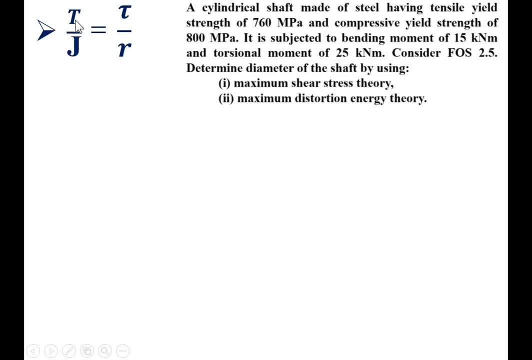 given to you torsional moment: 25 kilo newton into meter. so i can put it over here. so it is 25 kilo newton. so that's why it is 10 raised to 3 meter is converted into mm, so it is 10 raised to 3.. j is the polar moment of inertia and for the circular cross section. you know that. 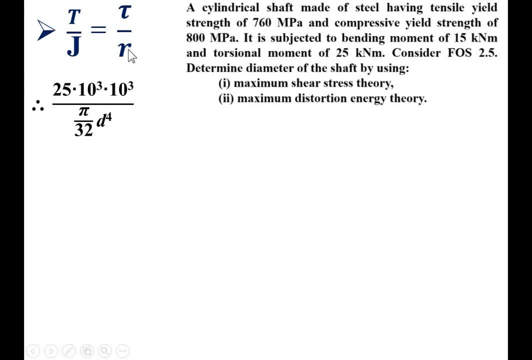 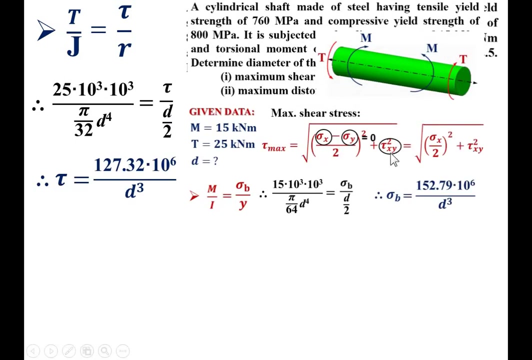 polar moment of inertia is pi by 32. d raised to 4 is equal to, as it is tau. that is my objective. so if you simplify this equation, then you will get shear stress in terms of diameter. so now i can use this equation tau max, because of now we have sigma x and tau both. 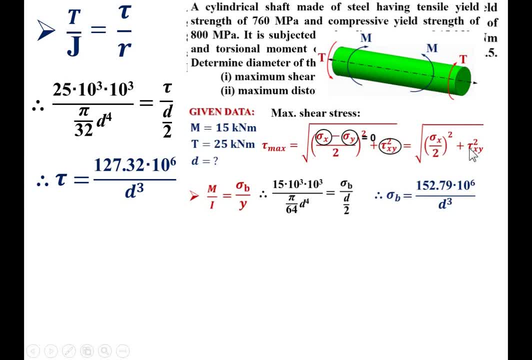 from this equation i can say: tau maximum is equal to this one. so now i can put it over here: the radius is equal to diameter by 2. so if you simplify this equation then you will get shear stress in terms of diameter. put it over here: the value of Sigma X and tau. so Sigma X, that is this one. 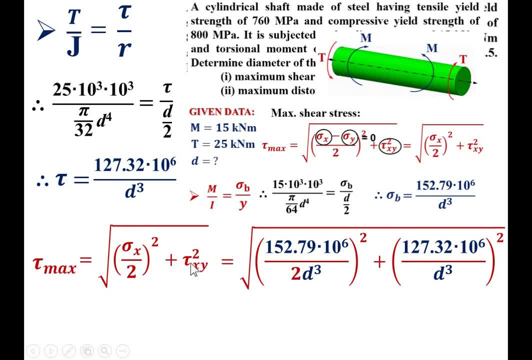 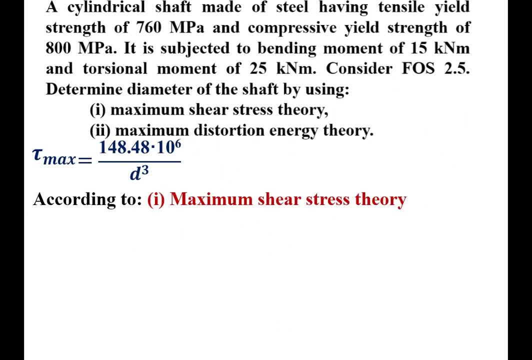 divided by 2, as it is plus shear stress tau, that is this one whole square. if you simplify this, then you will get maximum shear stress in terms of diameter. so once you got that tau max, then I can use the first theory. according to maximum shear stress theory, tau max is equal to 0.5 syt upon NF. so put this: 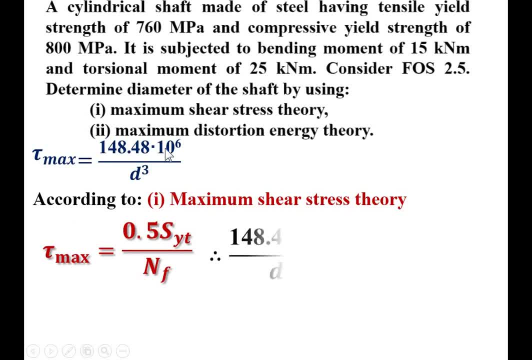 value tau max is equal to this one is equal to, as it is 0.5, as it is syt. that mean yield strength in tensile and that is given to you. yield strength in tensile, 760 divided by NF, that means factor of safety, that is. 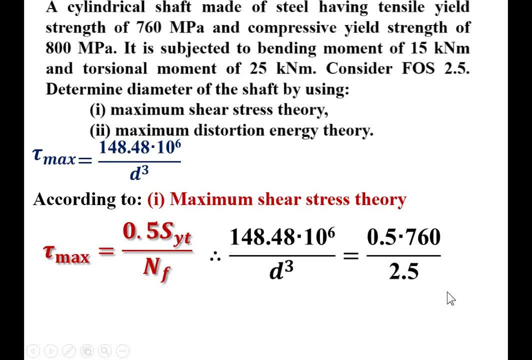 also given to your 2.5. so if you simplify this equation then you will get the diameter of the cylinder. so first you will get D cube and cube root of this one, then you will get D, that is 99.22. that is nearly equal to. 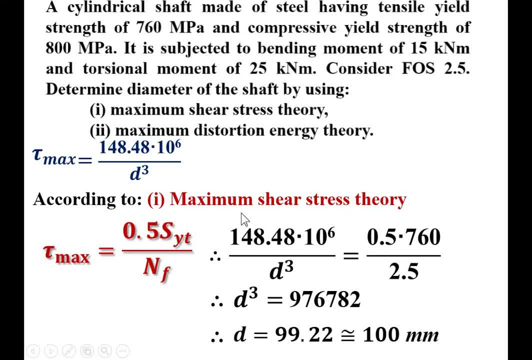 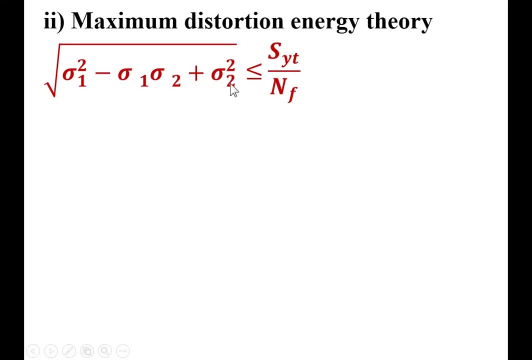 100.2 mm. so this is the first answer according to maximum shear stress theory. so make a box. now we'll go for the second one: maximum distortion energy theory. this is the statement of the maximum distortion energy theory, but here, unfortunately we don't know at this stage. Sigma 1 and Sigma 2. that means maximum principal.